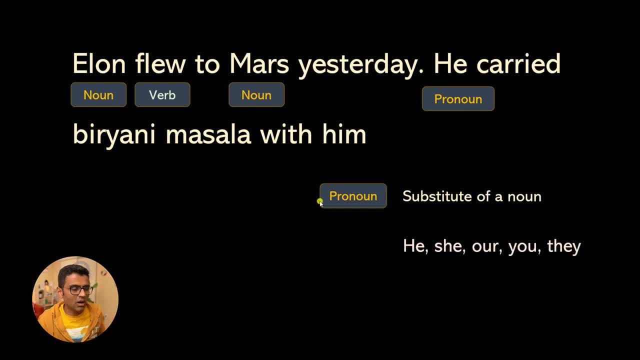 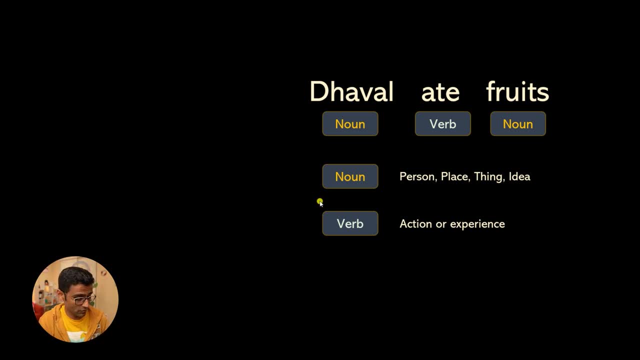 It's a substitute of a noun: He, she, our, you, they. all these are pronouns. Now, instead of saying double ate fruits, I can say I ate fruits. So in that case double is a noun, Whereas I ate fruits. 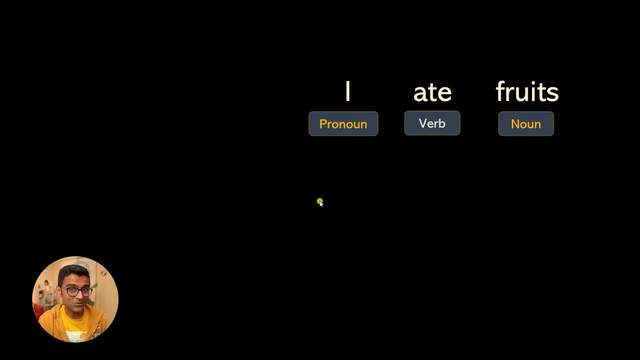 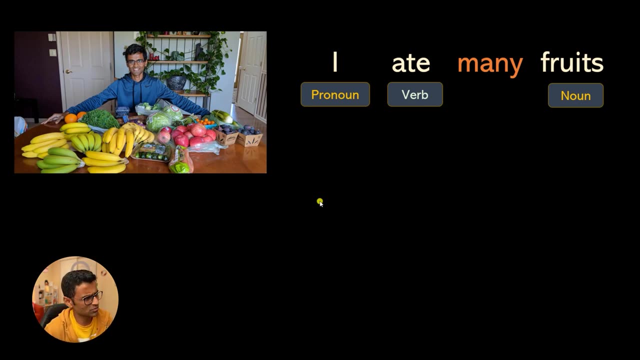 I ate fruits Is a pronoun. I can also say I ate many fruits. This is a real picture. by the way, I used to eat a lot of fruits when I had some health issues. I wasn't fruits for like three months. 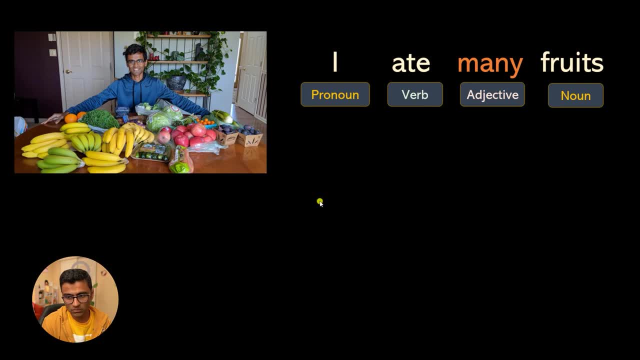 Here. many is called adjective because it describes the noun, adds a meaning to it. I ate fruits, But how many fruits? You can also say: I ate sweet fruits, or I ate citrus. ate citrus fruits or I ate tropical fruits. all these are adjectives. 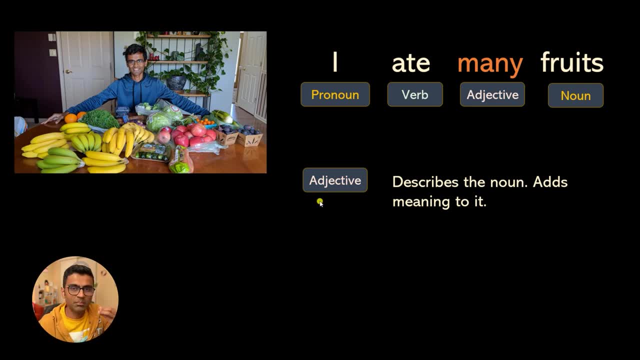 adjectives will add a meaning to a noun. here the noun is fruits, so it describes the noun a little better. I can say I bought Tesla. or I can say I bought red Tesla, so red is an adjective. smart engineer- crack the interview here. I have a typo here. but basically the smart- the word smart is an adjective- I want to. 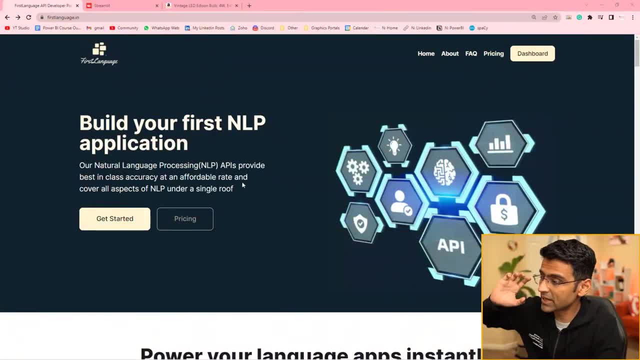 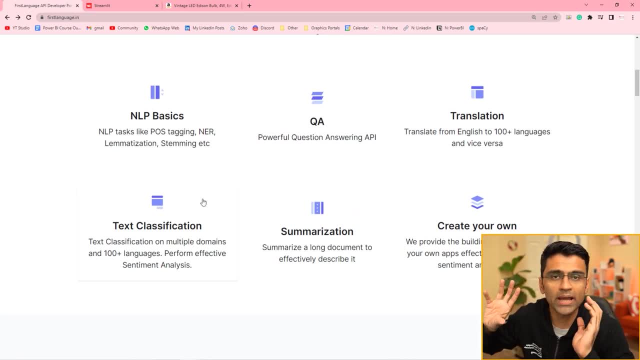 take a moment and talk about first language dot, in, which makes building NLP applications easier for you. you can perform various NLP tasks, which are shown here, via this platform. if you're using a spacey type of library, you download it. you run your code locally. if you are training a heavy model, you need higher. 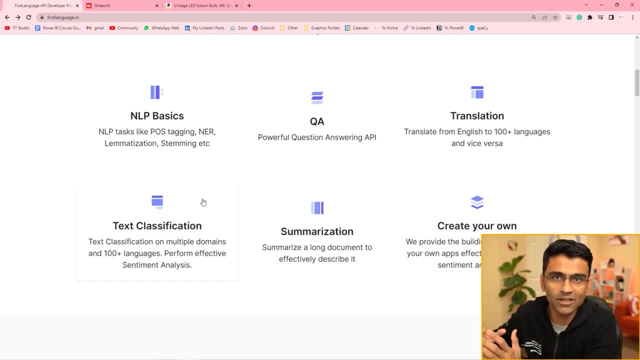 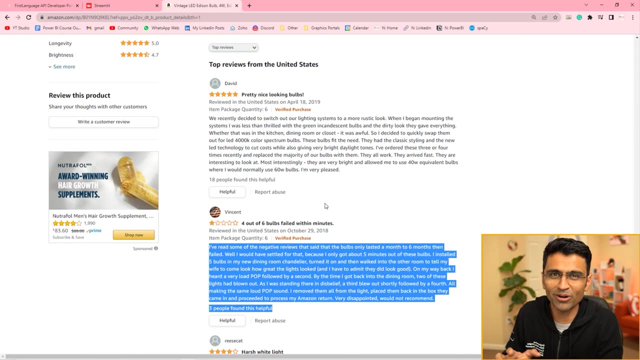 compute resources such as GPUs, whereas here everything is in cloud. you just make an HTTP call, things run on the cloud. you don't need a local machine with lot of compute resources. there is a demo which you can see by clicking on this link, and I have bought this bulb recently and you see there is a negative. 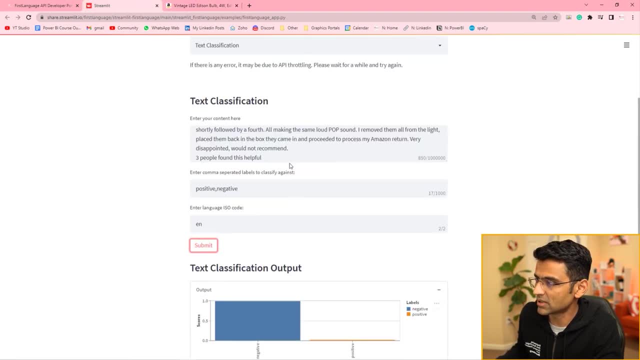 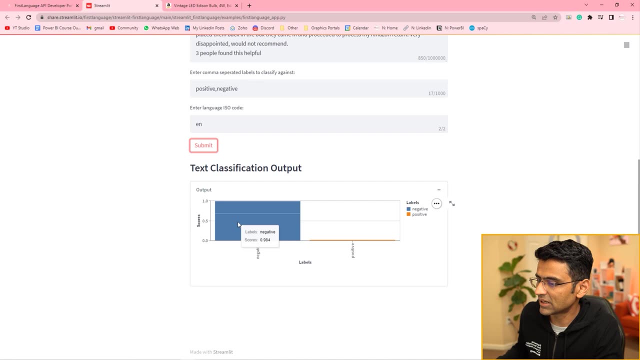 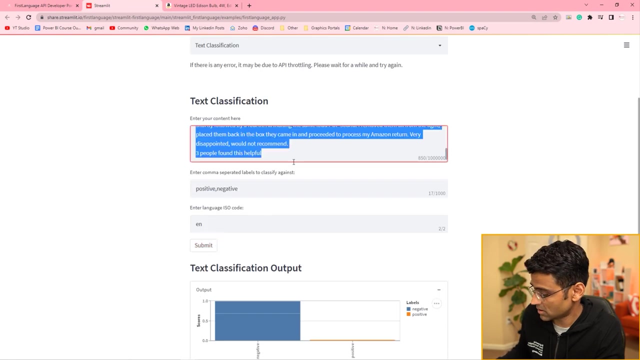 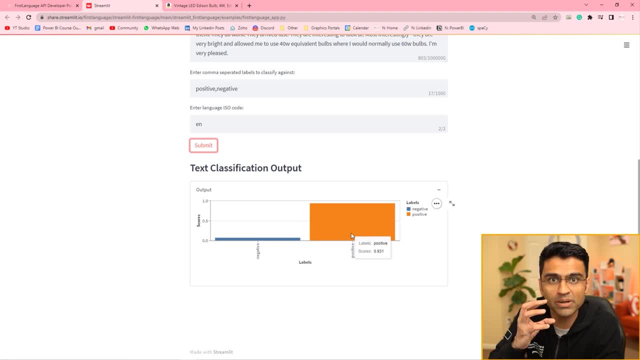 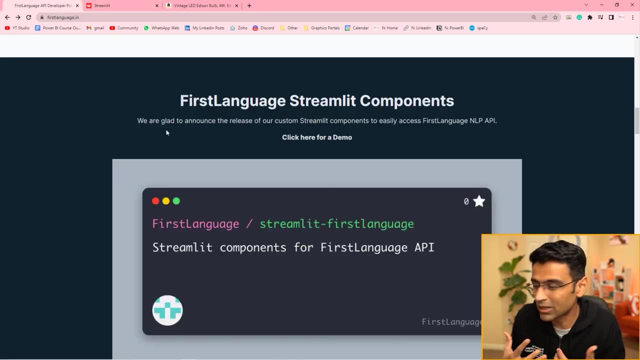 submit it, it will classify this as a positive. see, it's pretty powerful, so it makes things much easier for you. you don't need to have like too much like detail and NLP knowledge. you can just call a pi's and get things done quickly for yourself. the free time of the day is now up to you, so let's talk about the 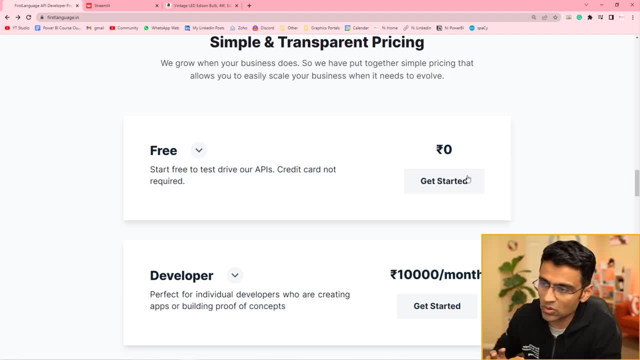 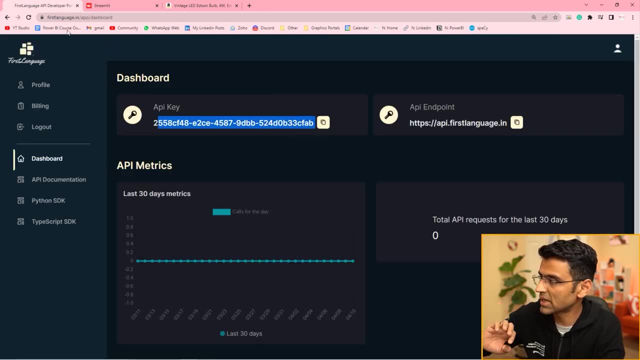 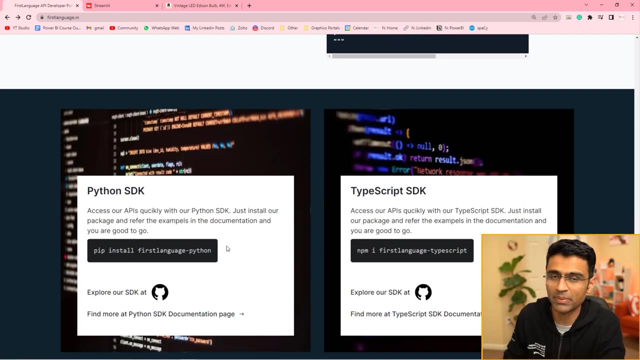 free tire is something you can try. today. you can just sign in and you can get an api access. once you sign in, if you go to dashboard you will get your own api key and you can use that api key to make the calls. they have sdks available both in python and typescript. go check it out. the 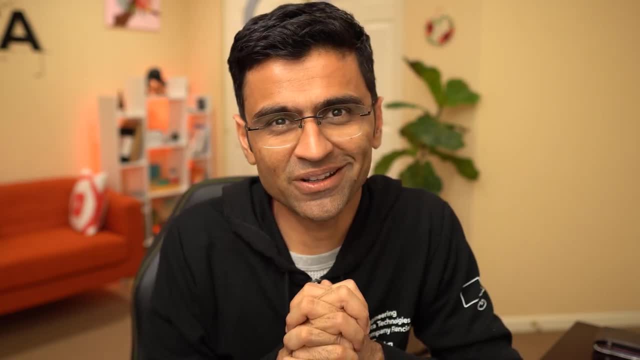 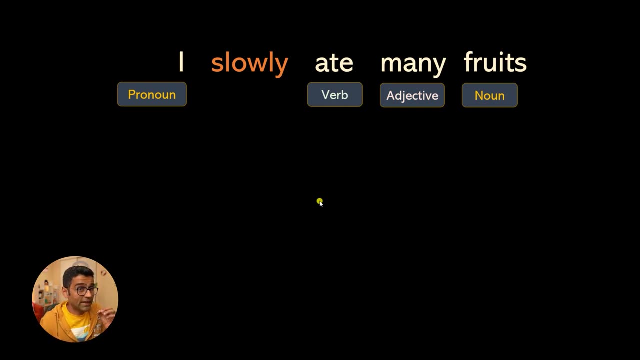 link is in video description below and thanks first languagein for sponsoring this video. how adjective adds meaning to a noun, similarly an adverb adds a meaning to a verb. so adverb is something that describes verb, adjective or adverb. i can say: i ate many fruits. 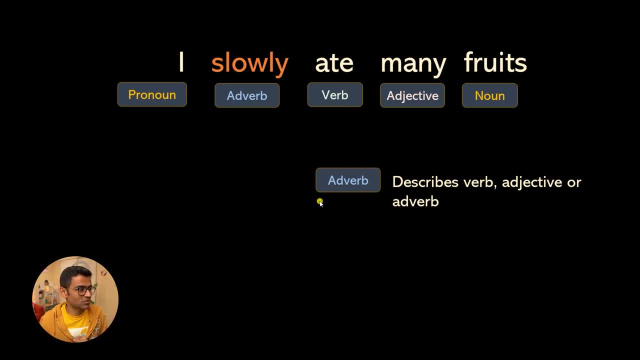 but now i'm saying i slowly ate many fruits or i quickly ate many fruits. you can say dog runs or you can say dog quickly ran, so quickly, slowly. all these are adverbs. they describe your activity a little better. they will add little more meaning to your activity, which is eating here or dog running. running is that. 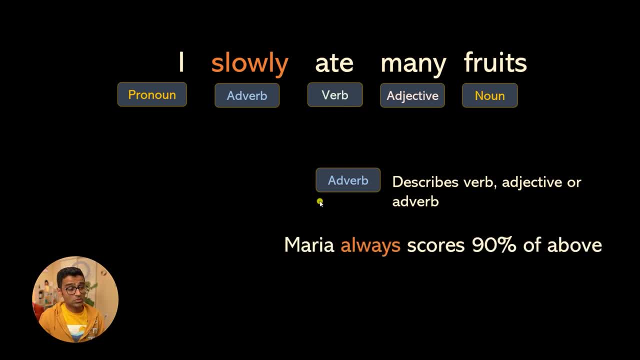 activity. maria always scores 90 percent of above. maria is one of those studious kids, so always is describing the activity of scoring. scoring is a is a verb here, but how? so you're saying always she gets 90 percent always. or we can say: maria sometimes scores 90 percent of above. so see: 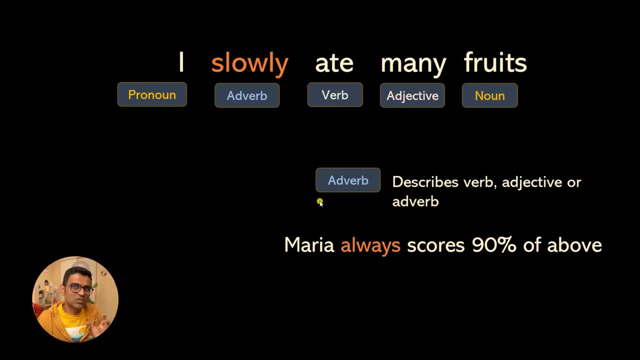 sometimes versus always, it's a different situation. she quickly learned nlp. we can say she learned nlp, but how she slowly learned nlp, or quickly, so here, quickly, slowly. these are called adverb and, by the way, these are part of speech. okay, pronoun adverb, verb, adjective. 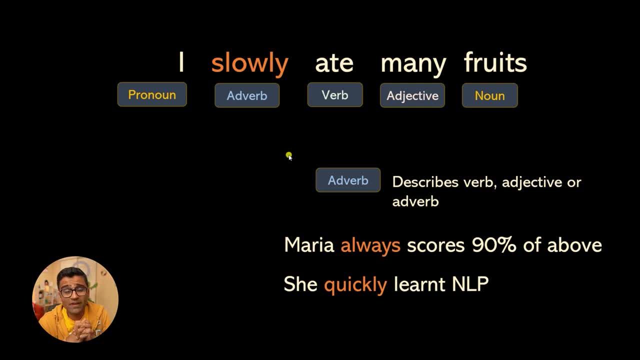 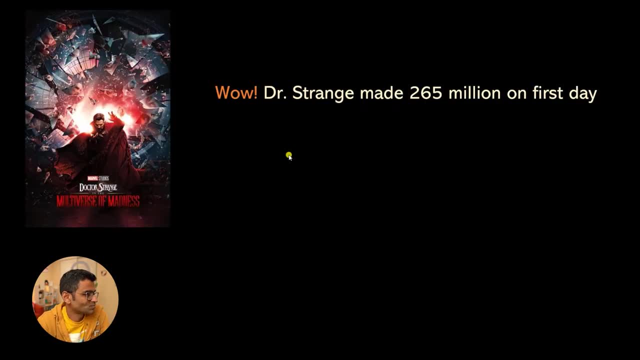 noun, if you google part of speech, you will find total eight part of speech. so we have covered few, let's cover one more. i'm gonna watch this movie, by the way, as my friends watched it and they really loved it. and when i was talking with my friends i was like wow, dr strange made 265 million dollar. 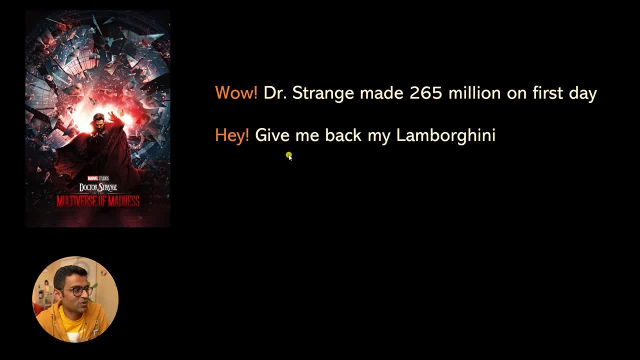 so the wow, you know the emotion that you have. you can say, hey, give me back my lamborghini. las he gotta know from google interview. so, hey, at last. wow, these are all interjection. they represent a strong emotion or an expression, you know. so those are called. 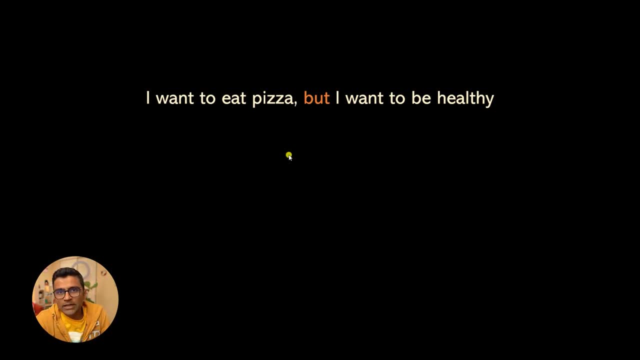 interjections. let's look at some other type of part of speech so you can have a sentence like this: i want to eat pizza, but i want to be healthy. hulk took a pen and started writing a story. do you think hulk can sit at a place and write a? 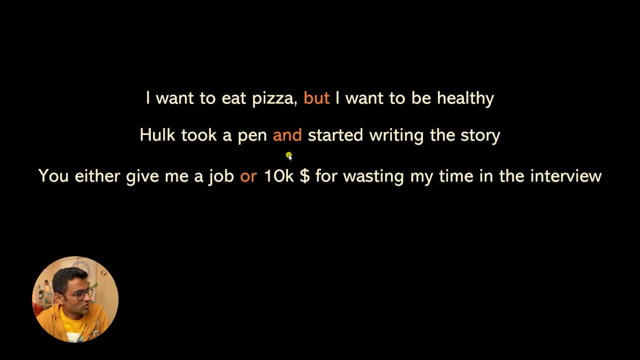 probably not. you either give me a job. you either give me a job of 10k dollar for wasting my time in the interview. here is a frustrated interview candidate asking for compensation for his six hours of time. but and or. these are connecting different groups of words and those are called 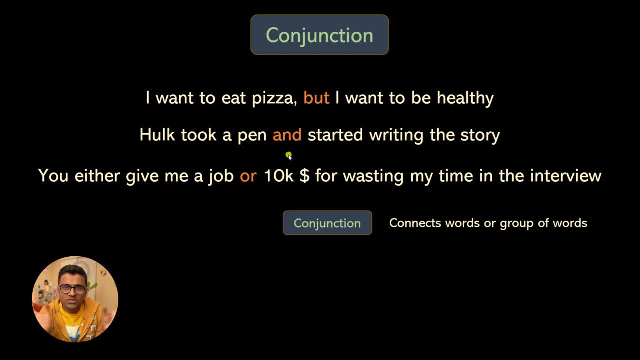 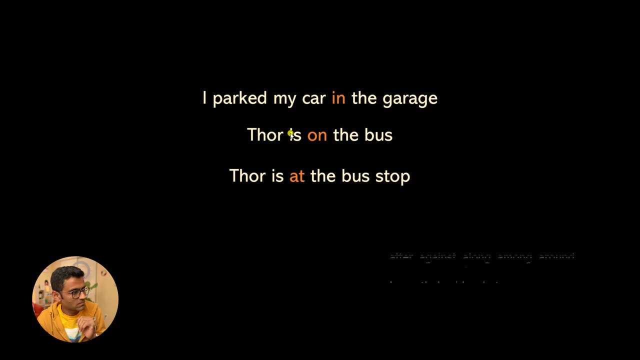 conjunction they just connect a group of words together. right here he took a pen- that is one group of words, started writing story, another group of word, and, and just connected them. so and, but, or, these are conjunction. then this is called preposition. it links a noun to another word. so 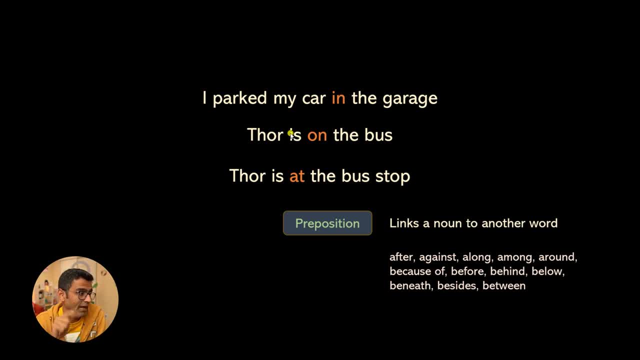 whenever you see: okay, thor is on the bus, or at the bus, or in the bus, see in on at there is a different meaning. so these prepositions are very powerful. they can change the meaning of the whole sentence. so they basically link a noun. so here, when I say thor is on the bus, thor is one noun. 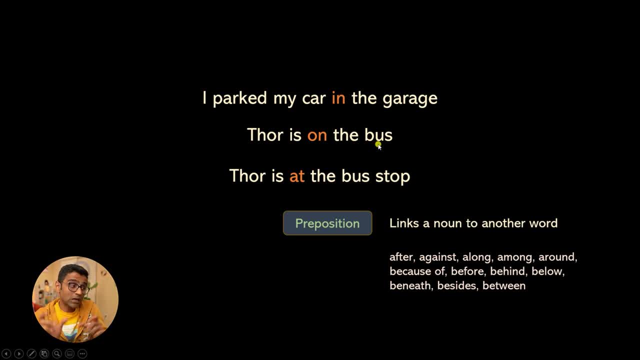 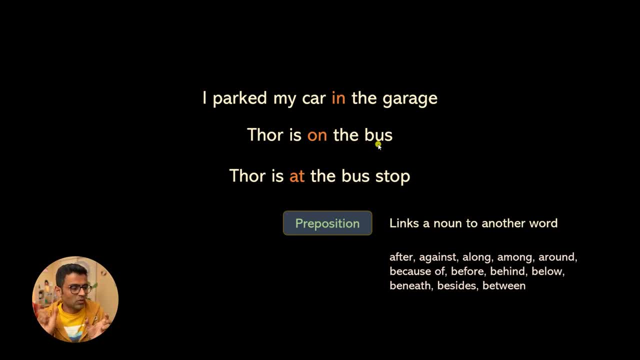 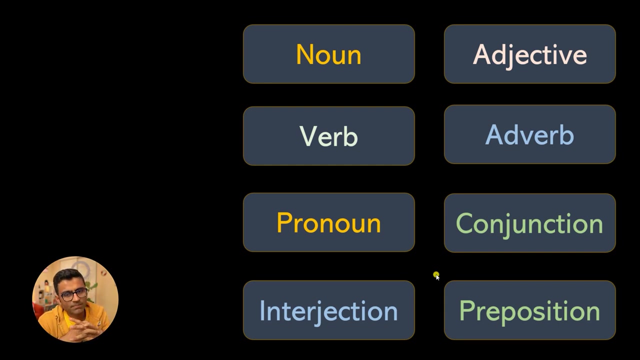 these are kind of connectors. they link a noun with another word and they're called preposition. so here are some list of prepositions. if you google preposition examples you will find a big list. so we talked briefly about these eight part of speech. you can google it like if you're. 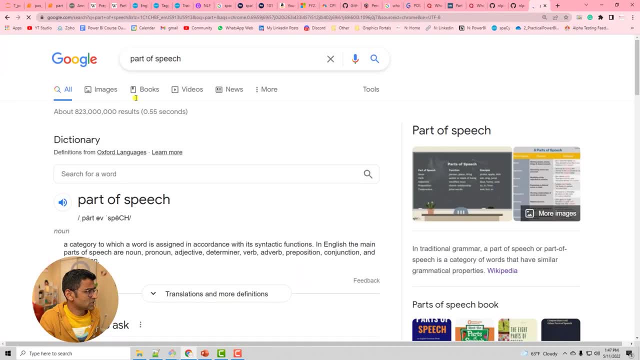 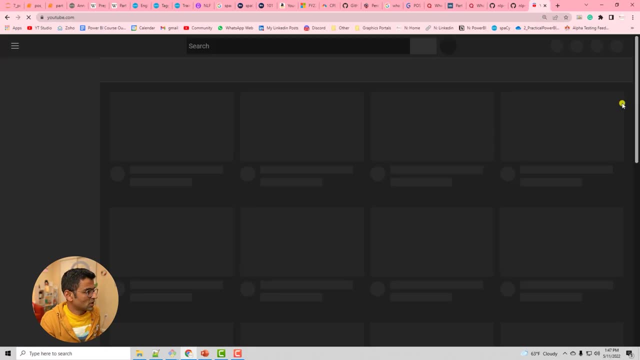 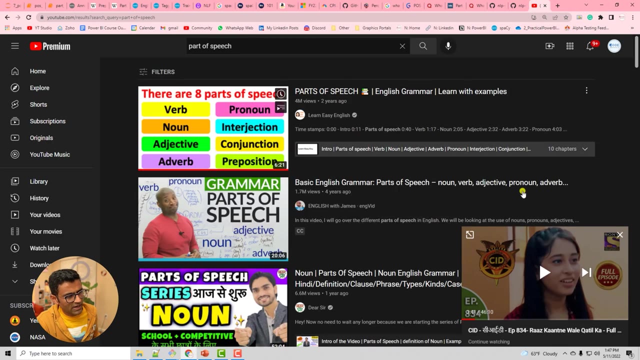 if you do google here and you do part of speech and you go to images, see, you'll find this is like basic english grammar. okay, nothing specific to nlp. you can also do part of speech, part of speech in youtube. you'll find n number of tutorials. if you're a native hindi speaker, i like 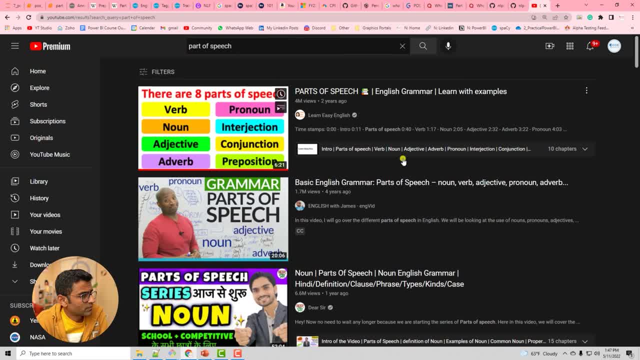 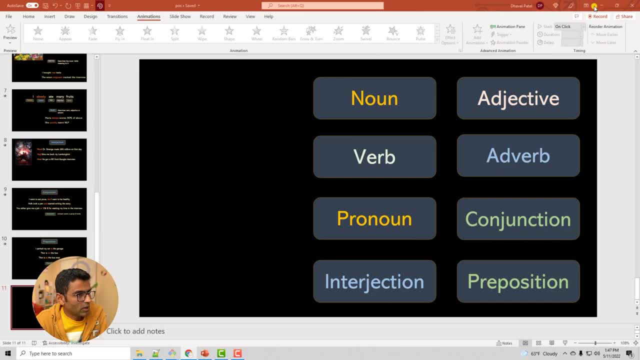 this, this person. dear sir, that channel is really good, so you can watch our videos if you want to know more details, but for now, I hope you enjoyed this video and I'll see you in the next one. bye, bye. now I'm interested in in the coding, so what we'll do is we'll. I have already launched a jupyter. 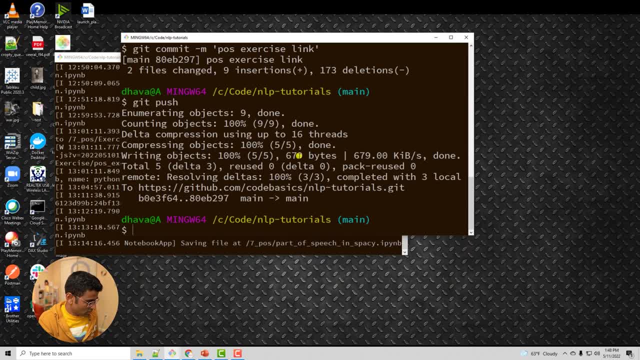 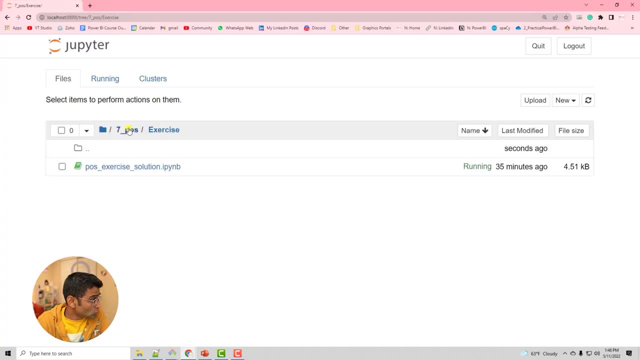 notebook. so if you have not, you can run this jupyter notebook command. it will launch a notebook. so let me pull that over here. so I'm going to create a new notebook here. so I have a couple of files, so ignore that, but I'm going to create a new. 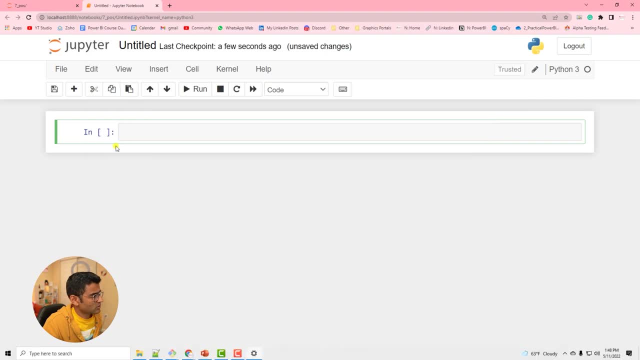 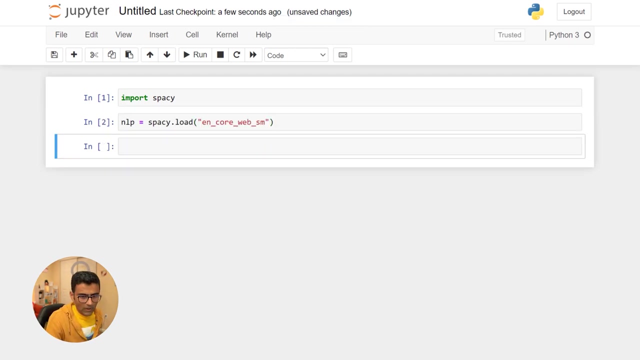 python notebook book and import specie from that. okay, so that's the first step. you do import specie and you load your model. so how do you load your model? like this, and i'm going to create a document with the sentence that we looked at and you can, you know. 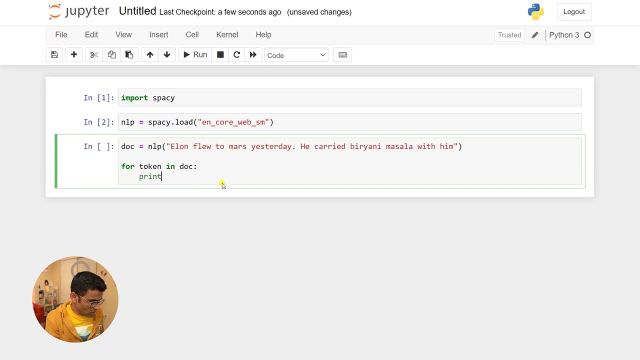 that when you do for token in doc, you can do something like this to print all the tokens. now how do you print the part of speech for each of these tokens? there's something called pos that you can use, and i'm gonna just separate them out. so 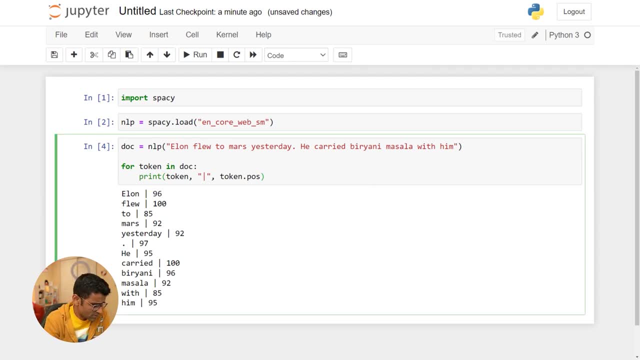 pos will print just the number. but if you do pos, underscore. now see, elon is a proper noun, it's a noun. but when i say i or a person, it is just a noun. but proper noun means a specific person. so when i say elon, that is a proper noun. when i say person, a person, right person. 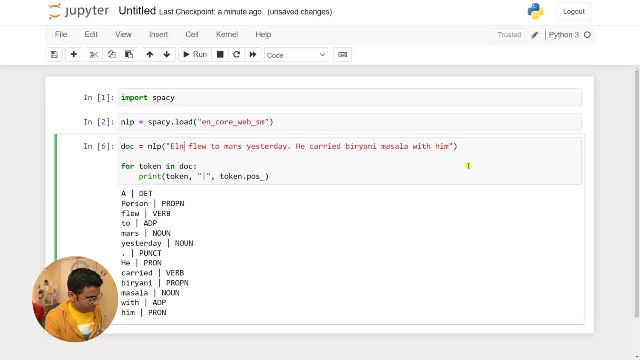 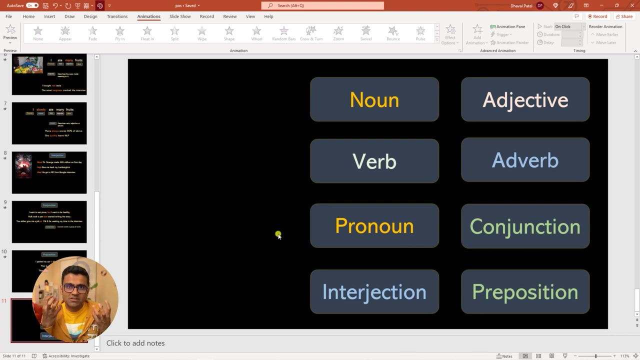 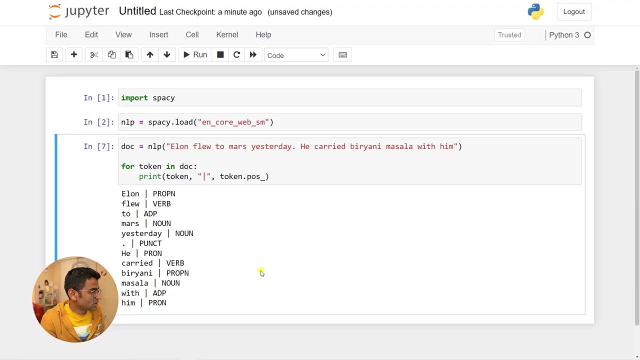 okay person is also a noun, so you will notice one thing, which is the pos tags that you see here. they are not exactly eight which i described. these eight are the fundamentals, the english grammar adjectives, some. sometimes there is some confusion, for example, if you look at okay part of speech article. 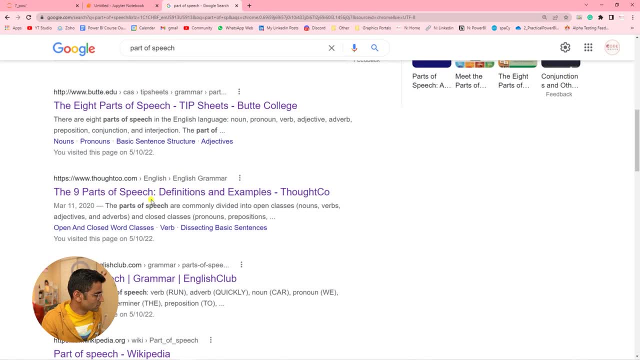 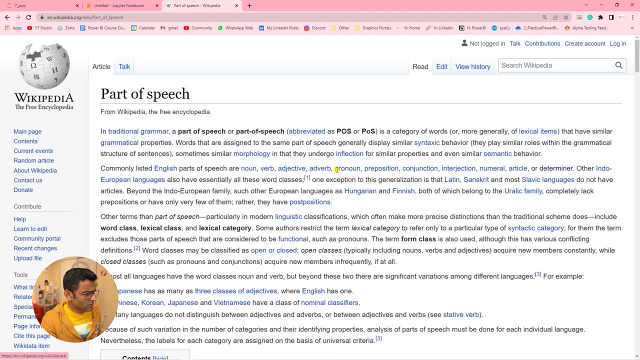 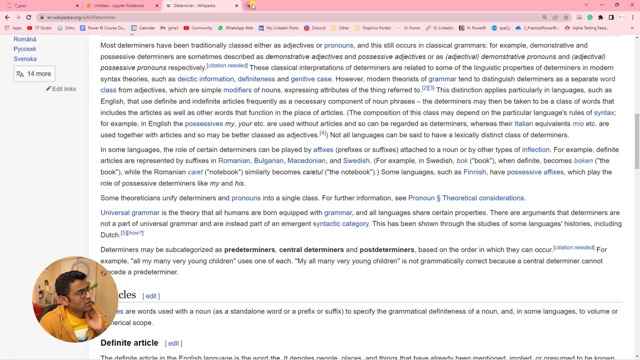 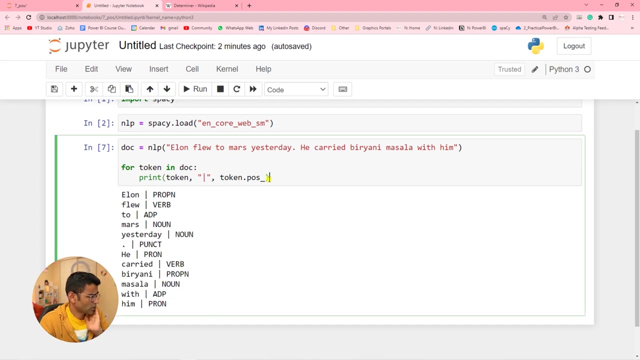 unless a Wikipedia- see here- it will say 1, 2, 3, 4, 5, 6, 7, 8, 9, 10, 11. so now here there are a couple of more, which is numeral article and determiner right, so you can say, okay, we will look into it. so here what you can do is let me just 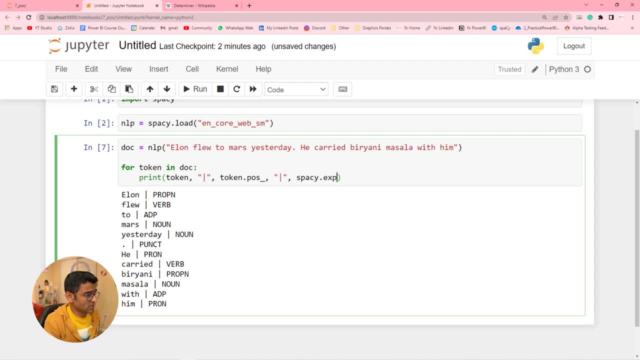 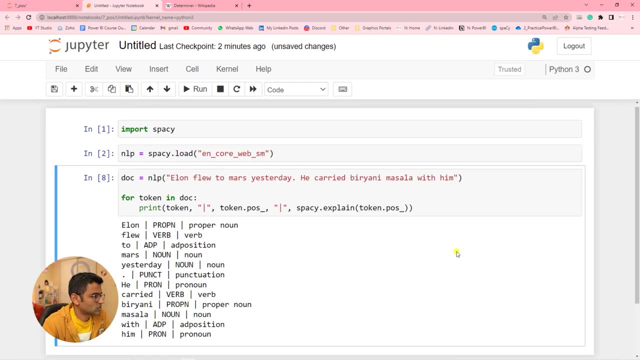 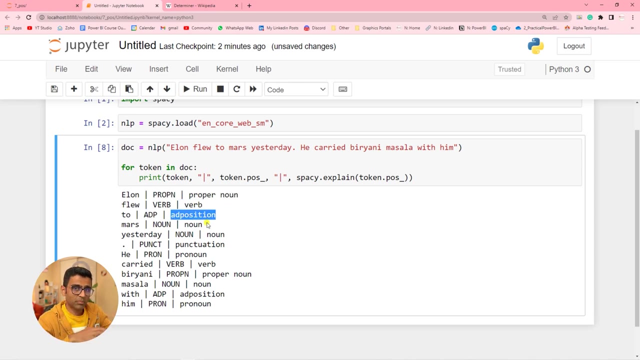 print some more information. so there is something called spacey dot explain, and you can give your pure stag and it will explain you. so instead of the just a code word, it will say proper noun verb now to is at position, it is. this is a preposition. 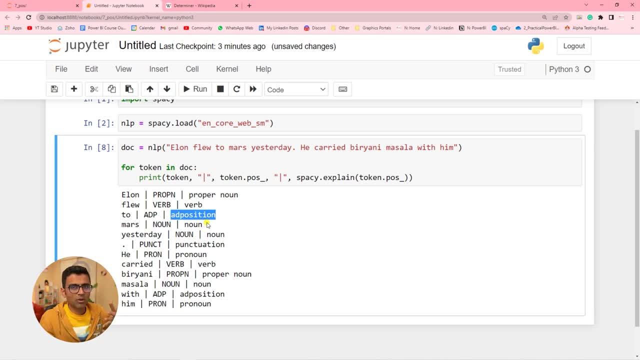 but at position is like a bigger group. there is something called preposition, post position, and at position is like a upper level. okay, that's why I'm saying what species? printing here is not exactly the same, but you're getting an idea. okay, so this is how you can print the part of speech and that explanation. 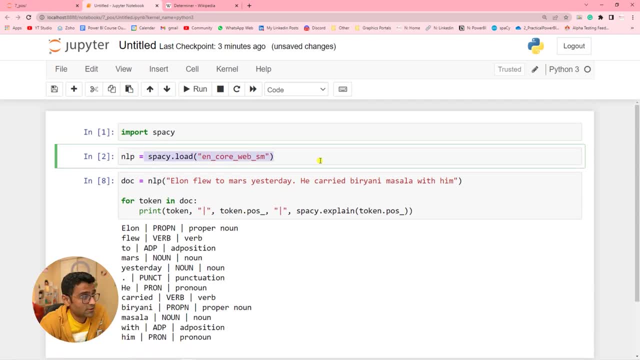 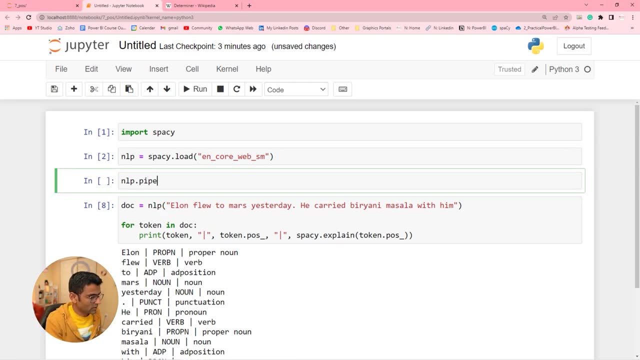 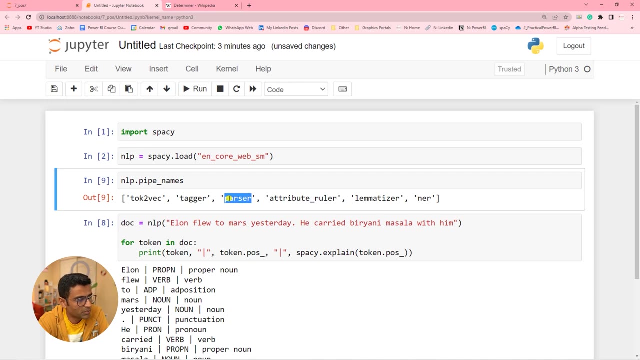 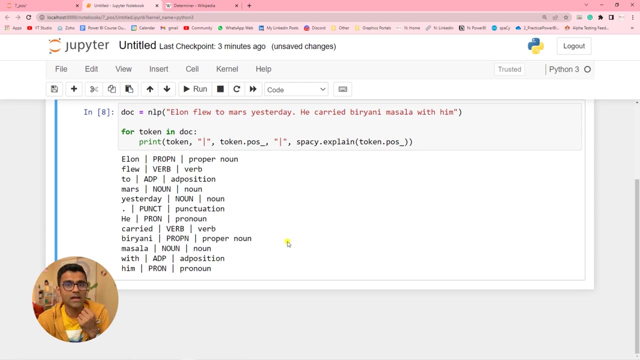 is PC. when you load this English train model, it will create a new string and it will give you the information about the text itself. so you don't have like a separate component, but to give you the sort of information about what is before. right, it will create this pipeline and these other components. I 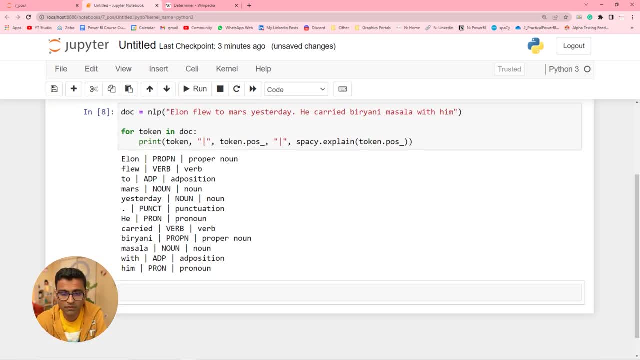 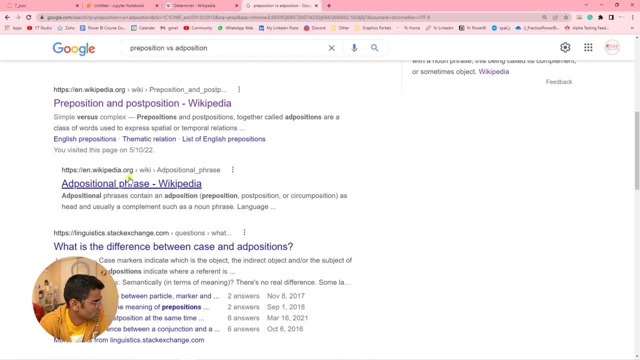 like a tiger parser. these components will create these part of speech. so you and I want to now show you a couple of articles so you might be confused about pre position, pre position versus at position. so there is a, there's an article. I I'm gonna link all these articles. as I said, this is not a an. 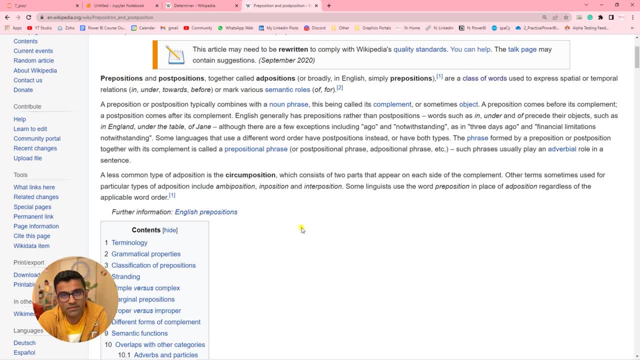 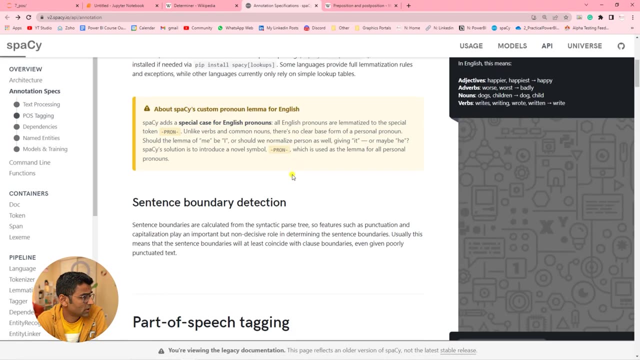 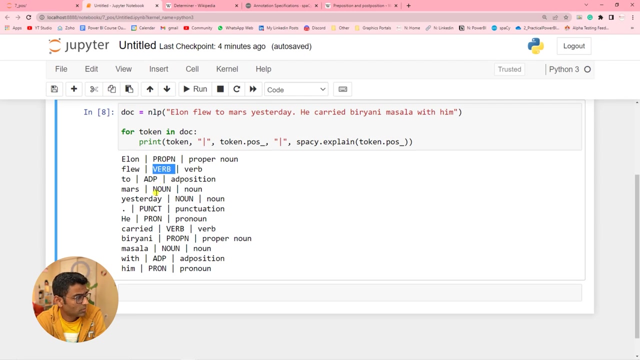 English grammar tutorial. if I try to cover English grammar, this, this is gonna be a big video. so I will cover all these articles, just in case you have any questions, and here I'm gonna link this particular documentation as well, where it is mentioning all the text. so here we saw right proper noun verb punctuation. 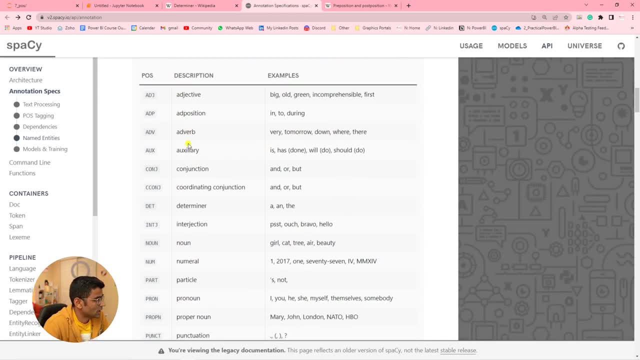 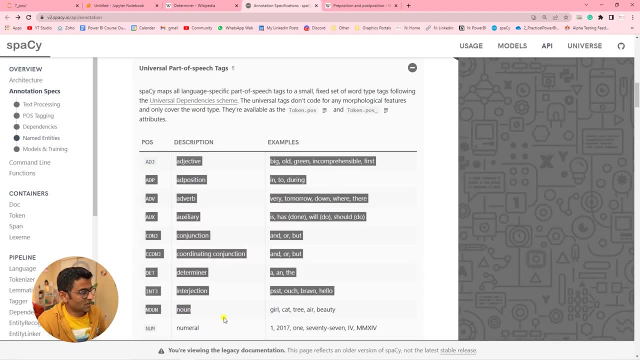 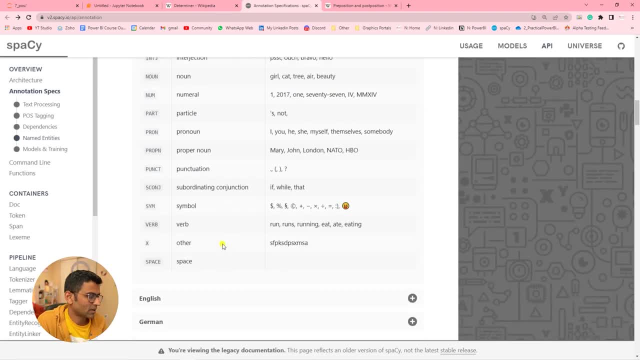 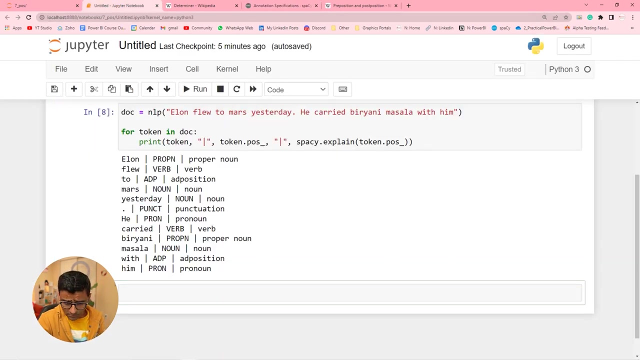 eight. see, there are so many of them because they are doing sub categorization. there is thing, something called other. if you have something garbage like some other token, there is something called X. now, that X is not part of that eight POS tag that we saw in English grammar, but that's okay. so now let's take a different. 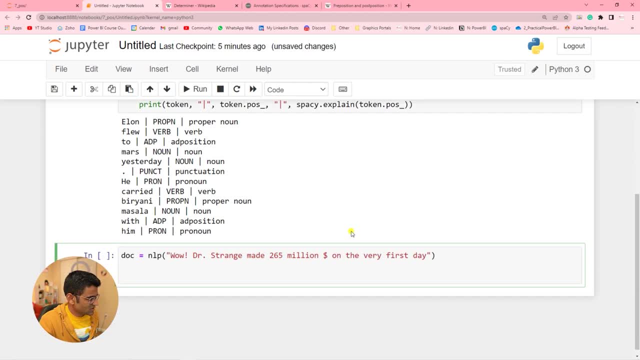 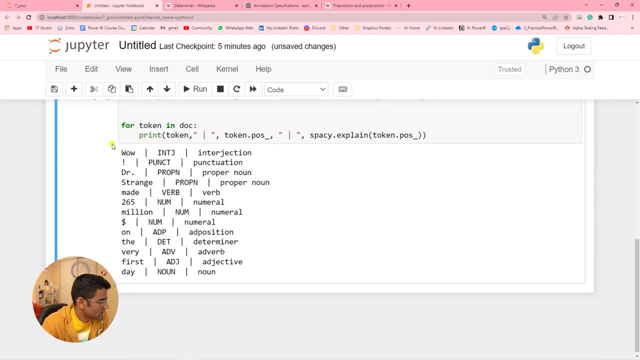 example, talk. strange, you might have seen this movie already, and if I, but in same thing see wow is a interjection, then this excellent exclamation mark is a punctuation. made is a verb. okay, now one question: made is a verb, but it is a past tense, so is there a way that I can know this is a past tense? good news is there. 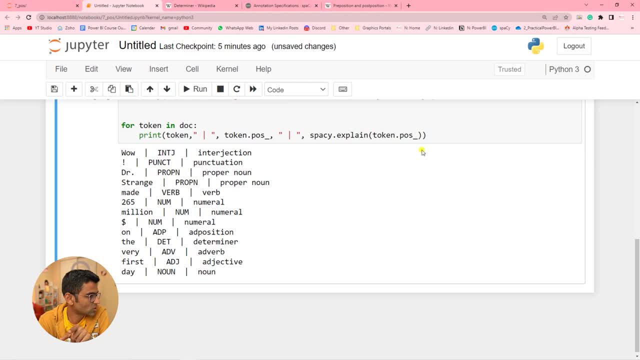 is a way. there's something called tags. so if you print a tag, so let me print it here. so I'm going to print something called token dot tag and see for made it printed VBD. now what is VBD? again, you can use PC dot. explain for this thing: token dot tag. 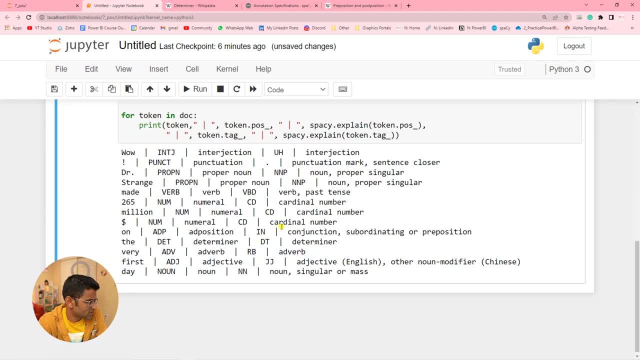 and you will notice it says verb but past tense. so tag underscore is nothing, but it's a further categorization. it's it has lot more details than what POS contains. okay, so that's what the tag is. when you have a numeral, it says cardinal number. when you have 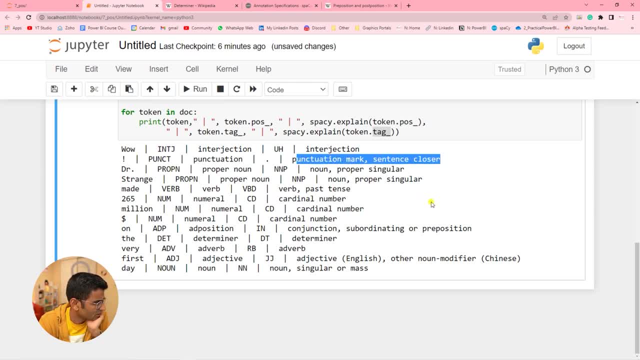 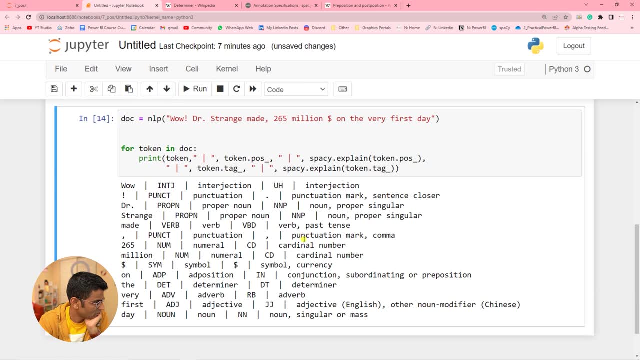 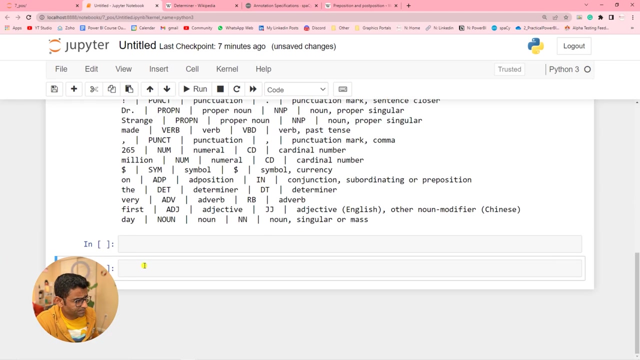 see punctuation mark. it says sentence closer, correct, if you have a punctuation mark such as, let's say, comma here. so here it says punctuation mark comma, and here it says punctuation mark sentence closer. so it gives you little more detail than just the POS tag. now see, you'll realize that space is kind of smart and it can understand. 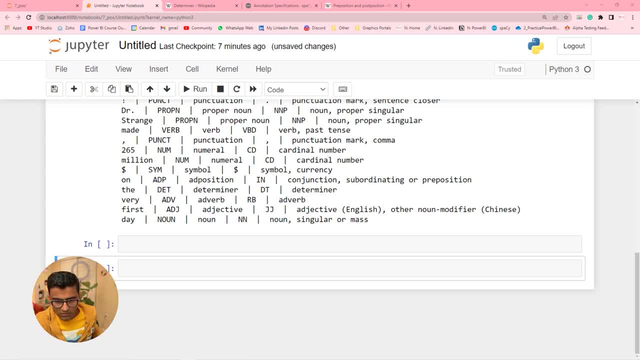 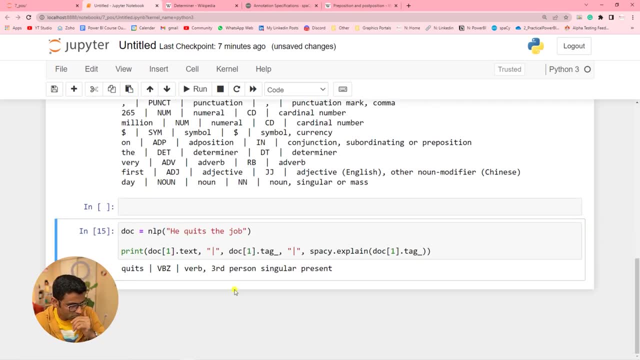 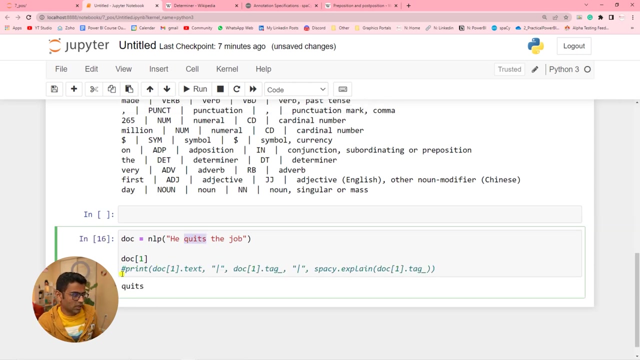 whether it's a past tense, present tense, we already saw. but let's look at one more example where you have this sentence: he quits the job. so here doc one. so okay, so doc one. when you look at doc one, let me comment this: doc one is quits okay. and if you print doc one, dot text and tag. 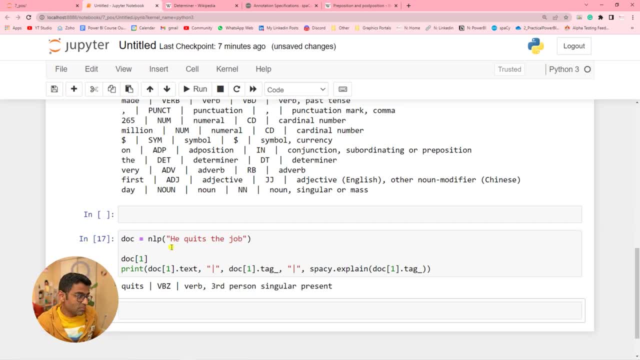 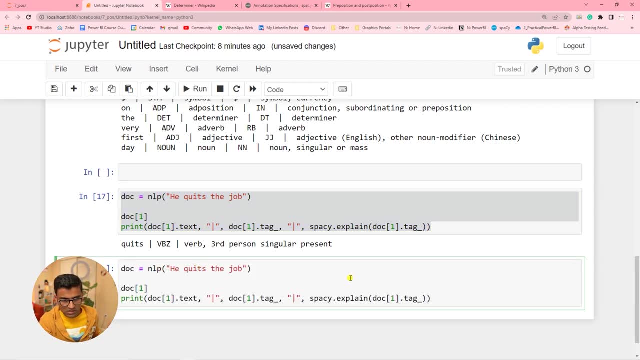 okay, third person singular prison. so this is in present tense. but what if I change this and I just say he quit the job? say I'm just removing s. now it knows that this is a past tense. when you have s, it's a present tense. see: third person prison. here it says past tense, so space. 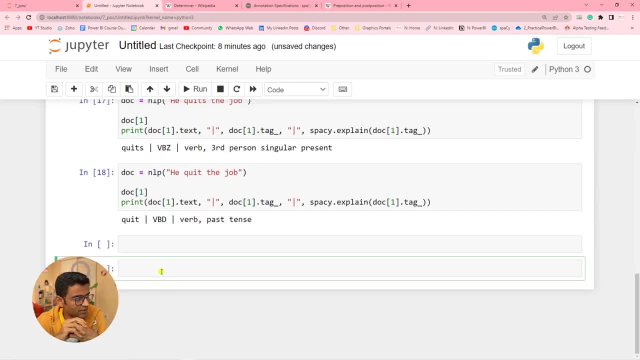 is smart enough that it can figure out whether, what kind of tense it is, and you can already see the application in. when you're building NLP application, knowing this kind of information, having these tags, is gonna be extremely useful now. now let's do something fun. so I want to open Microsoft's earning report. 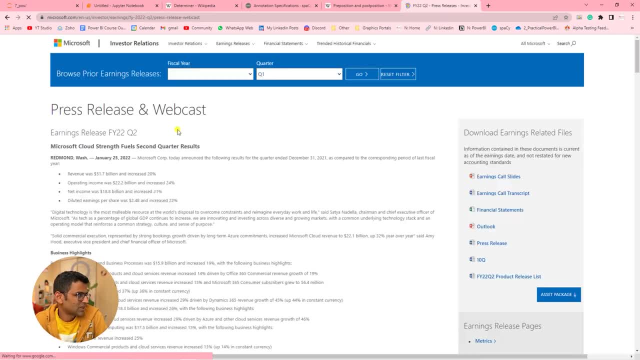 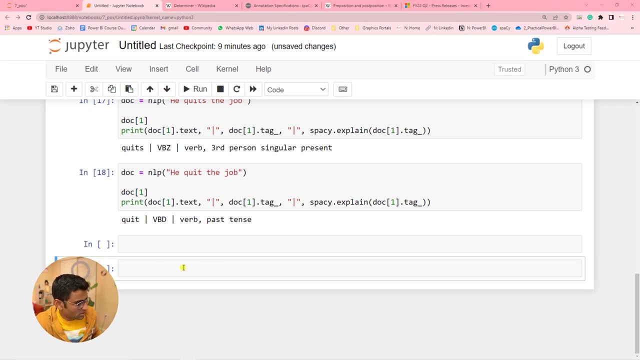 so all these big companies, you don't display their earning report, basically the quarterly performance, and I want to grab the text from this earning report. let's say, I get some of these, these text, okay, so you just say copy and you paste that and you know that's a, that's a text, that text that I have. 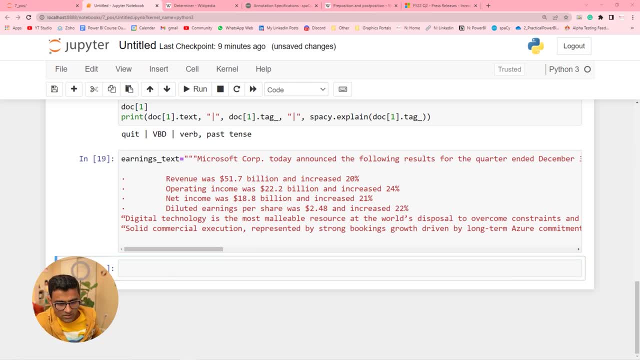 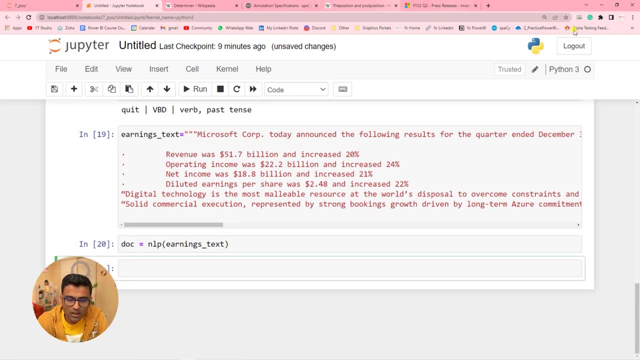 and I want to do some NLP analysis on this, so I'll create a doc out of this text. okay, and one of the things you want to do potentially is you want to remove all the punctuation marks and all the extra characters from it. for example, if this had a character like I'm just 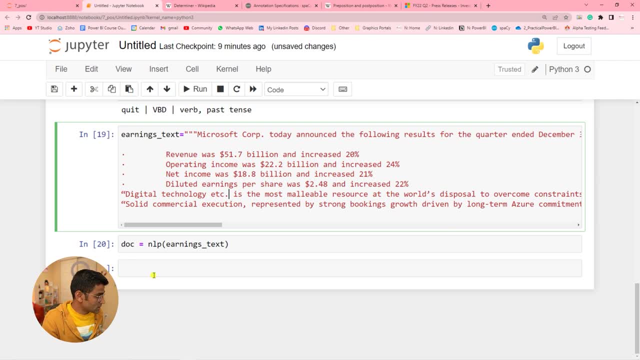 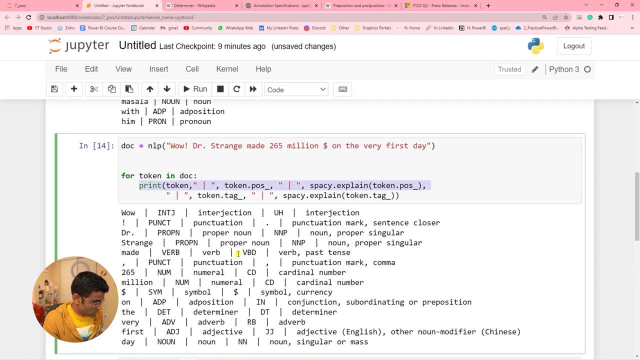 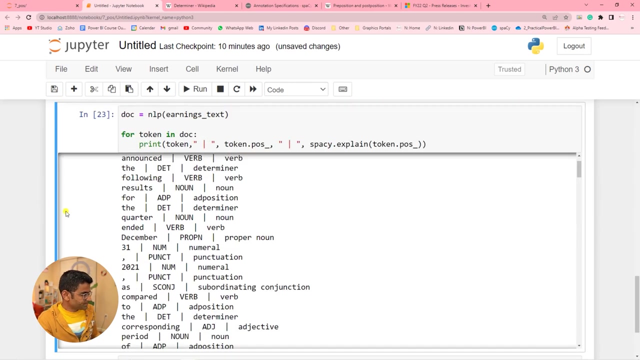 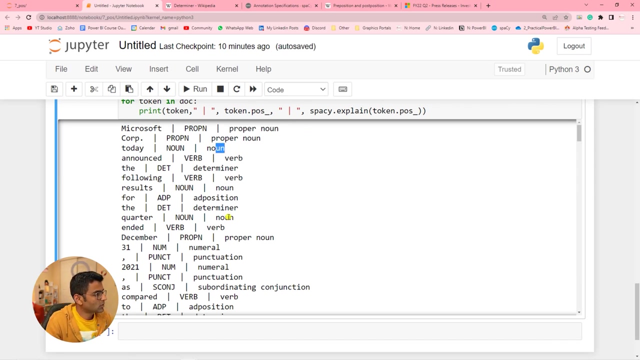 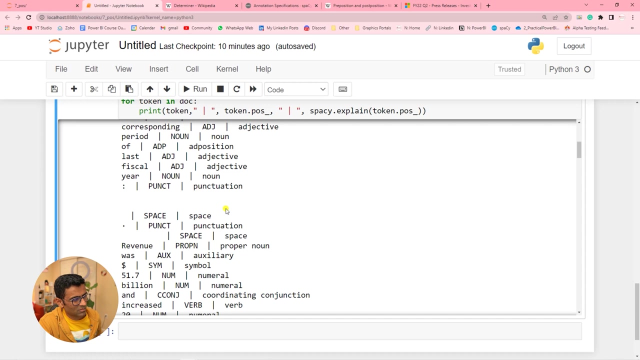 putting, etc. etc is one of those extra characters and if I have something like this I can support. you can print the POS. okay, so you can print. and you will notice that while you have proper noun and noun, you also have things like space, for example. spaces is not useful, maybe based on the use case. you want to remove punctuation. 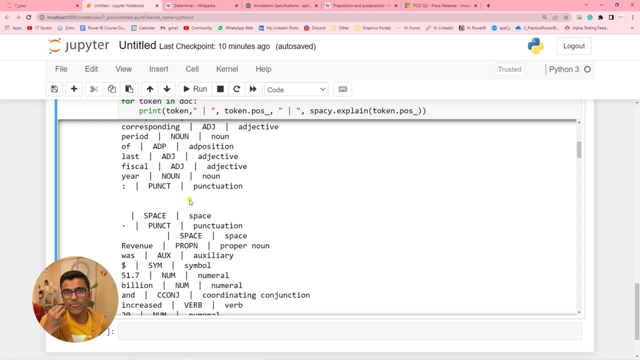 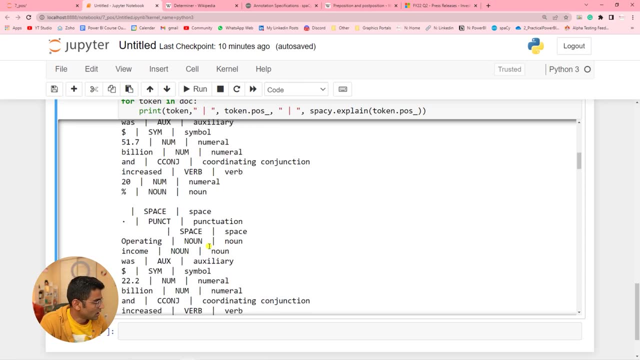 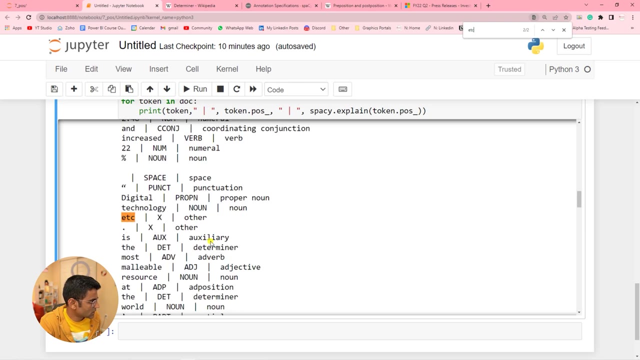 also, you want to get rid of all these extra characters so that you can perform some analysis, you can build some NLP application on top of this text you also have: let's see where is my etc. see the type of etc. is X, the POS tag is X, dot is: 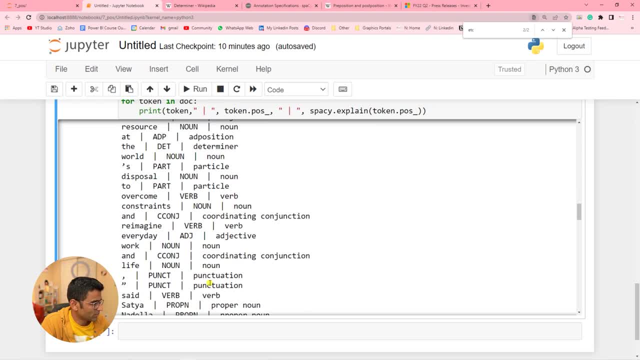 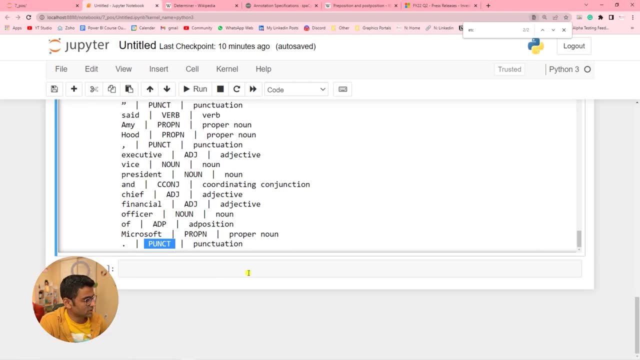 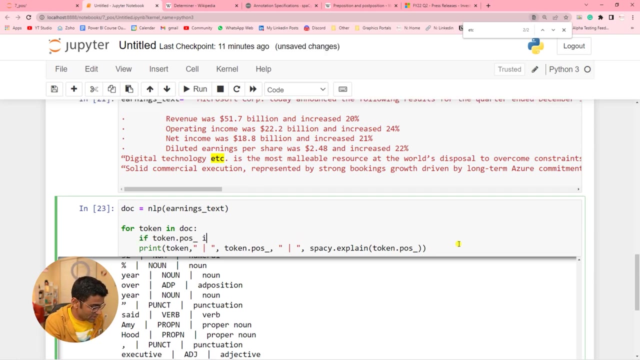 also X, and these are not useful, so you want to remove them. so how do you want? how do you remove them? so you have punctuation. so I want to get rid of all this. so what I can say I can do is I can say if token dot POS, in meaning if it is one of these. 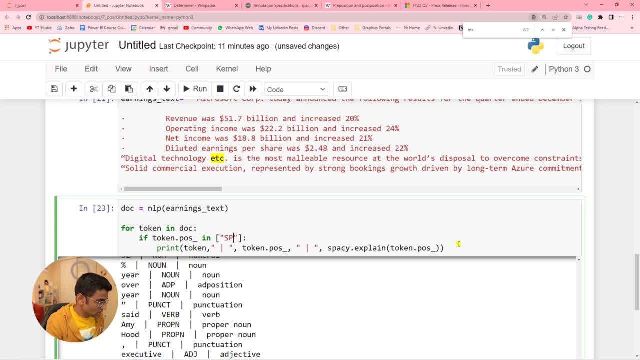 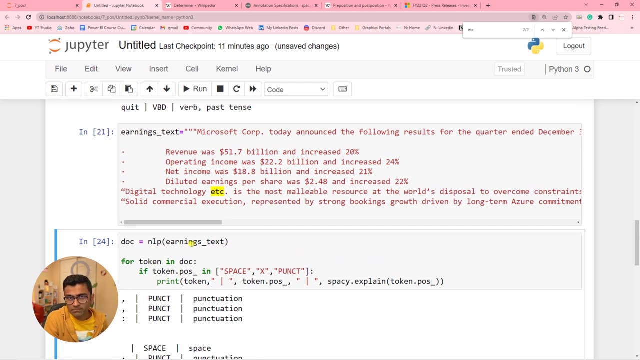 then remove it. so you can say: if it is space, if it is X, make, if it is punctuation, say: I have all these, these are all unnecessary character. I want to get rid of them. this see some of the punctuation, by the way, that might they might be necessary based on what kind of application you are. 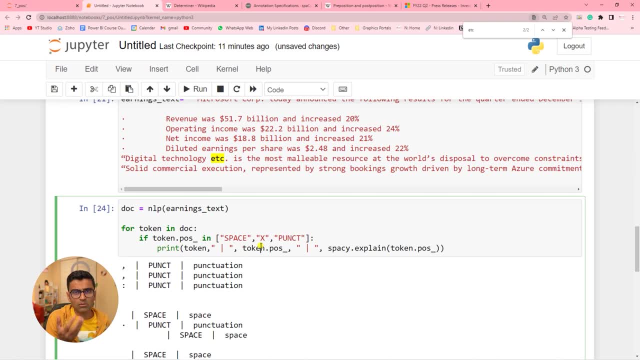 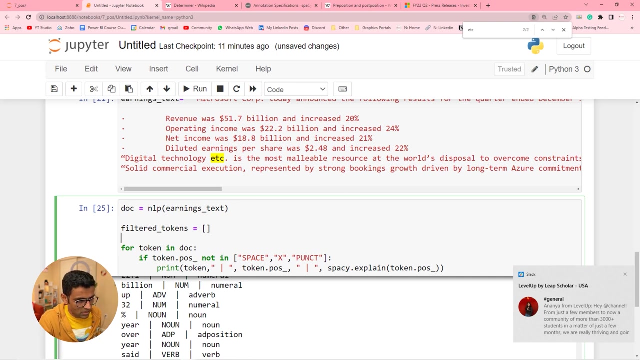 building. but I just want to demonstrate how exactly POS tagging can be used in a real world application so you can say: if this is, if you do not, you will get the reverse right. those tokens- space x punctuations- are filtered and you can save these tokens in, let's say here: 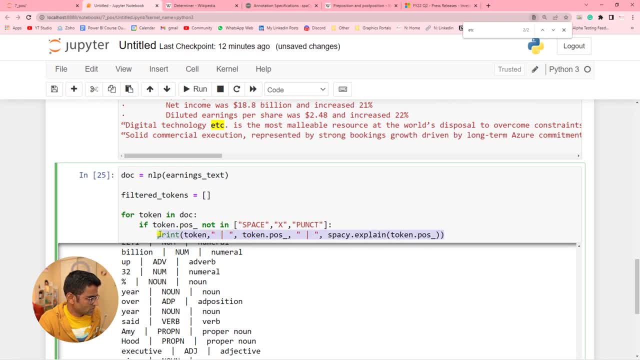 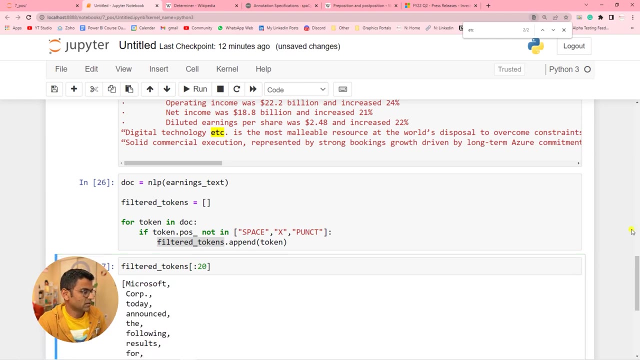 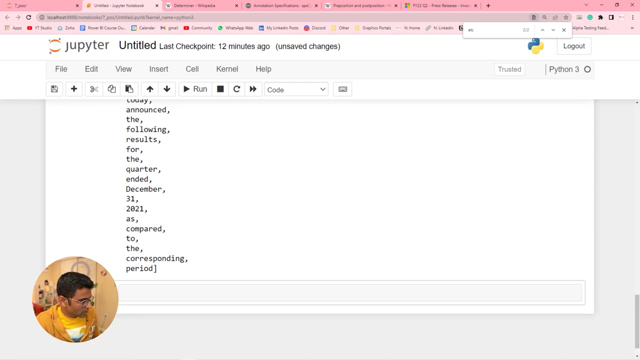 and you can just say: filter tokens, filter tokens, dot, append token, and then if you look at these filter tokens, you will find that all that garbage is been cleaned out. okay, now one other thing you want to do with, uh, this text is: you want to know how many nouns. 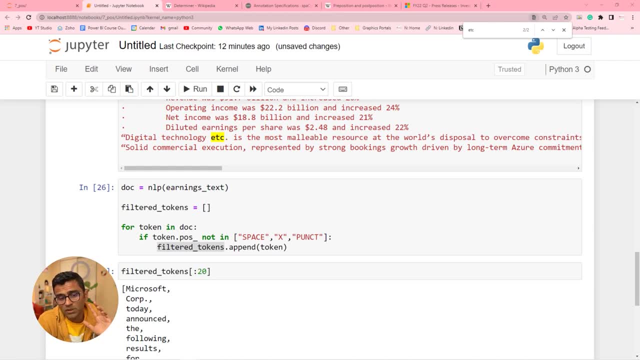 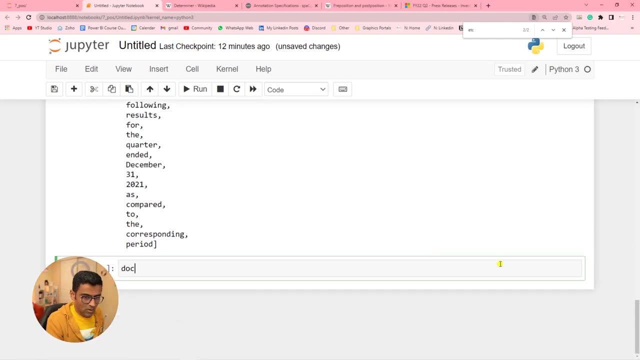 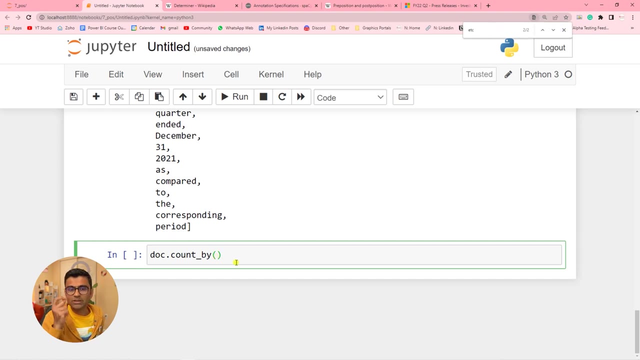 are present, how many verbs are present, and that could be one of the useful thing you can extract. so spaCy provides a convenient api called count by. so this count by will give you the count of all those tokens. so you can say: space, spaCy, dot, attributes, dot, see here, if you do dot, you can extract the count by for 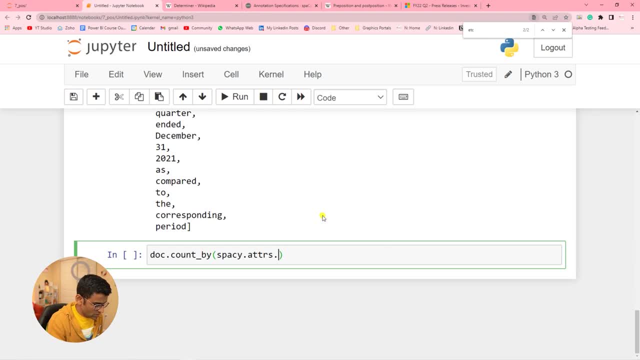 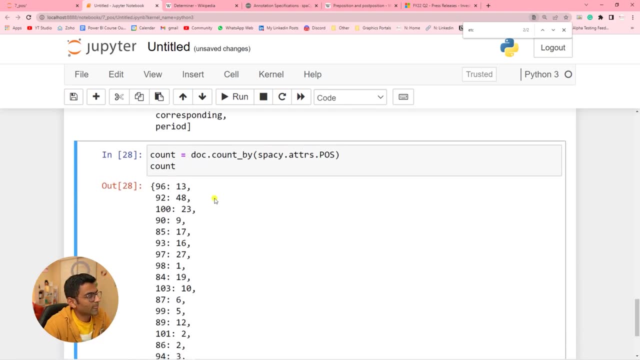 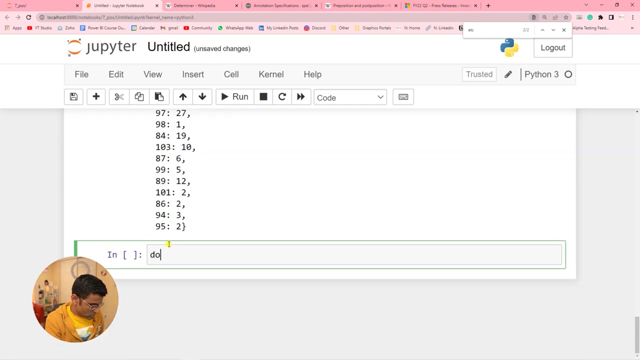 tags: posc. you can do it for pos. let me show you pos. and it is just showing you that pos 96 has 13 count. now, what is 96? well, let's, let's see so. doc, dot, vocab, 96, dot. text. so it is saying there are 13 proper nouns. 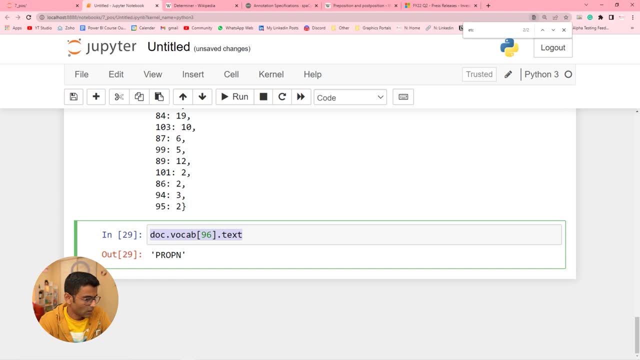 in the in the text and if you want, you can just- uh, you know it's a dictionary. so for key value in count dot items, this is a you might be aware about this basic python syntax that you can iterate through the keys and values of dictionary like this and you can print. 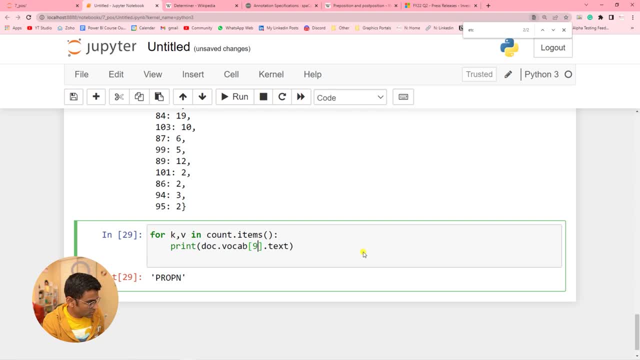 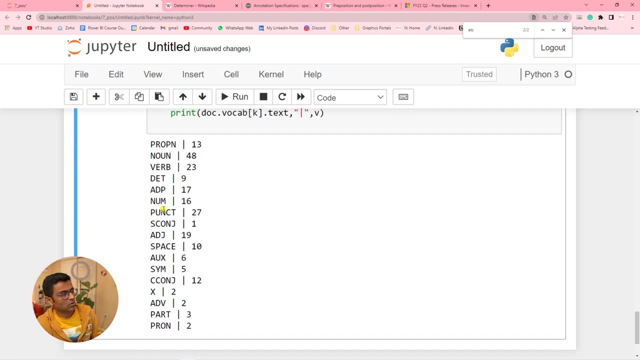 you can print what. so you can print what kind of pos that is, and something like this. so in this microsoft earning report, the paragraph which i get here today, that noise is probably this: Classy to the level language class on routine anyway. alt. add text to the text: dallas. and if you want to do it, you definitely need the dallas. 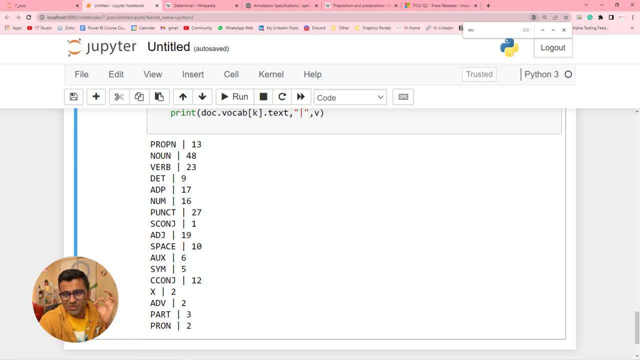 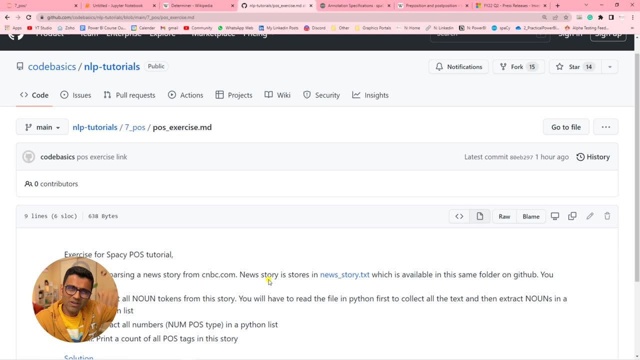 and if i want to do it ininku day ininku2, then just add text like you did, and your best interest is that. uh, if you want to add text in your, however, the completed text in the paper style format, you can either use your arms according to your purpose, and if i want to use 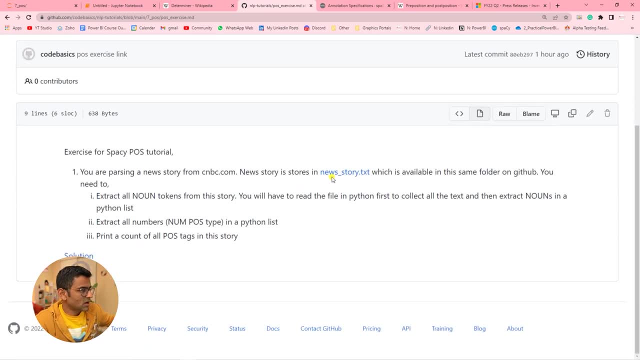 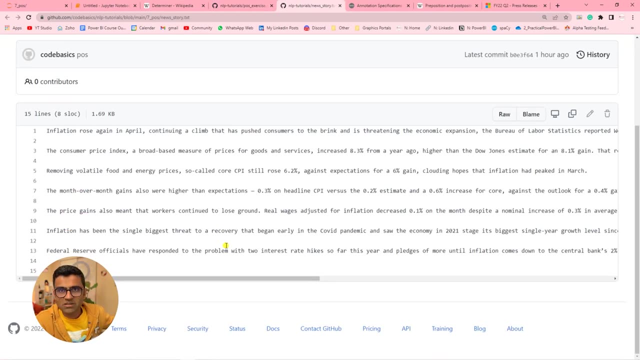 moto letters, for example. you can use the capacity add text in your normalizedrew and also on the. I grabbed a story from a CNBC comm. it's a story on info in inflation. inflation is rising so you need to extract all the nouns, then extract all the numbers print. 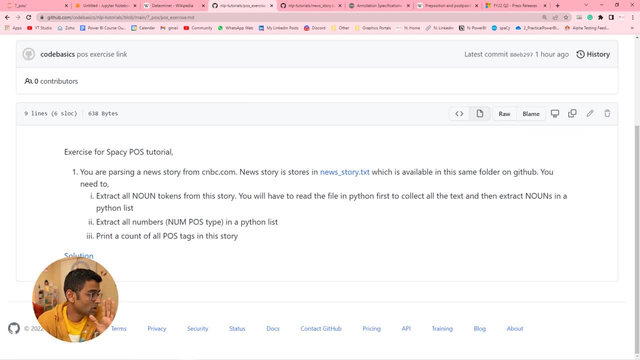 account very simple exercise. in the future I might add more exercises as well and if you are interested in contributing, all you have to do is add a new exercise along with a solution and give me a pull request on my github so you will find my github here. you can give back, but die days we want to have.